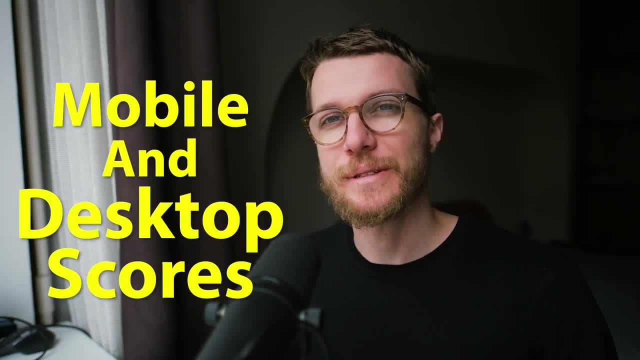 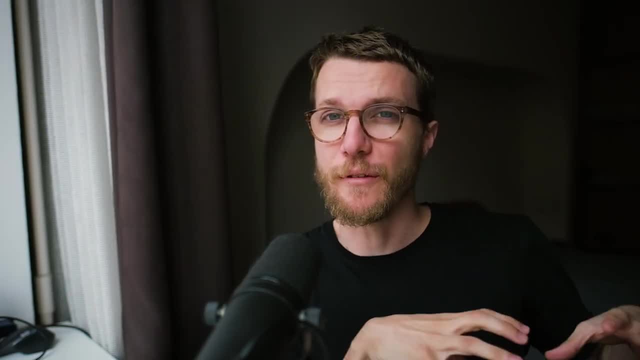 Chrome dev tools And this will measure both mobile and desktop scores, because a lot of the time they're different if a site isn't mobile optimized And you can augment your site with something like AMP to make it super, super fast. Anyway, like I said, if you're a freelance, 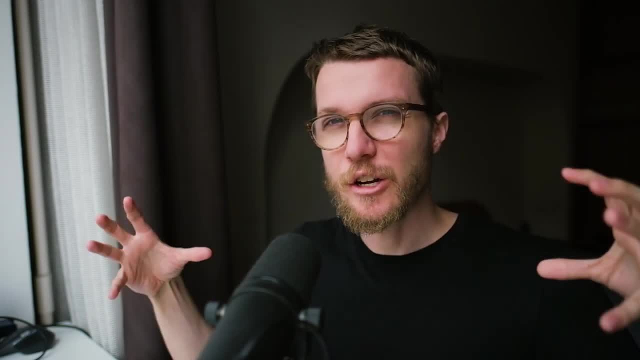 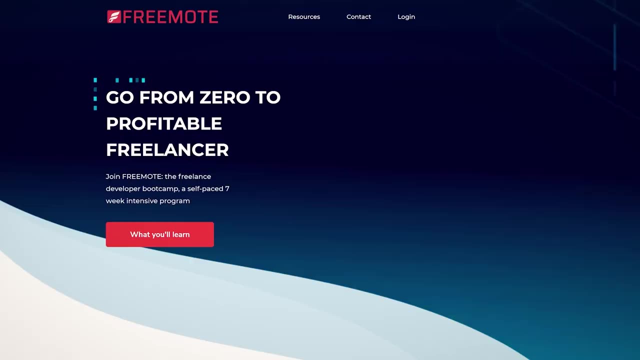 developer. this is a really, really good tool to use. So if you're looking for a site that's really powerful, service you can sell and you can craft an insanely good offer around this, for example, speeding up your site by 20% or it's completely free- Just a quick plug: we train freelance. 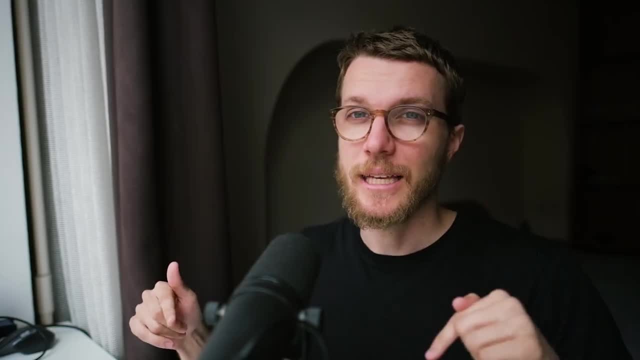 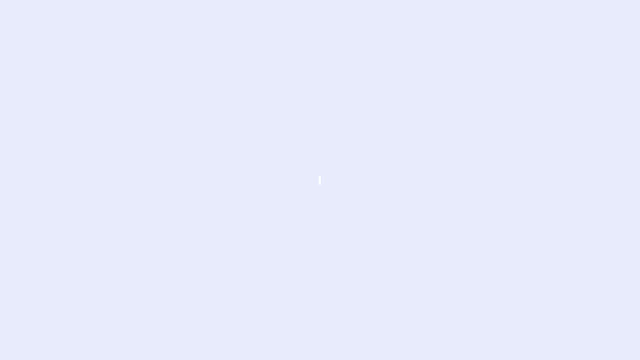 developers from scratch in freemote. the freelance developer bootcamp link below, if you're interested. Okay, now let's talk about fixing these issues. 10 ways you can actually speed up your sites after you've done your speed audit, And the first one is pretty obvious: you want to compress your images. 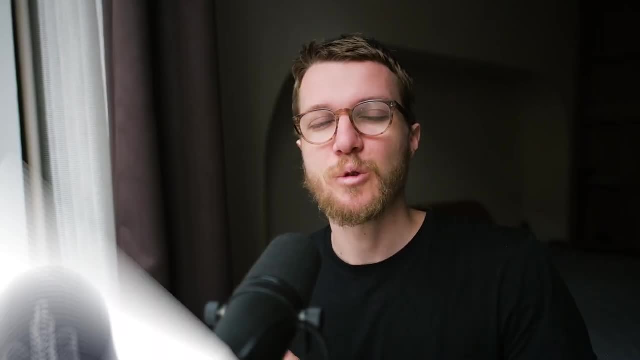 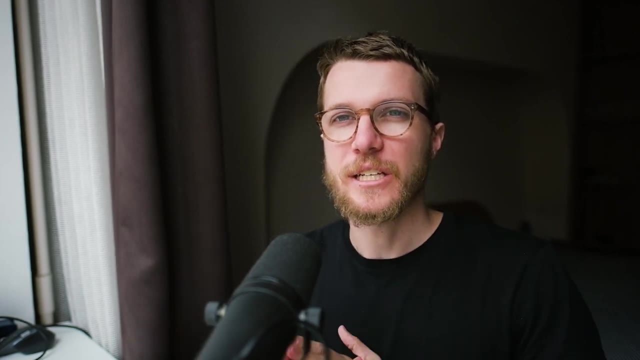 and iframe your videos. there's a ton of online compression tools. for example, tiny PNG is usually going to reduce your image file speed. So if you want to compress your images, you want to compress your image file size by up to 60% or more, And it's almost always better to use an optimized video. 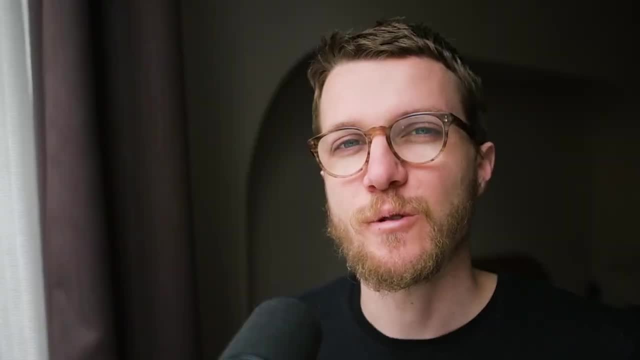 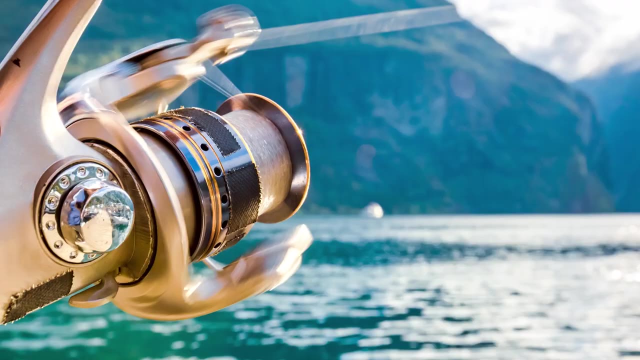 player like YouTube or Wistia, instead of loading the actual video files into your project. Beyond this, you want to make sure your images are the right size. you don't want an absolutely huge three megabyte image. you don't want a 2000 wide pixel image that's only being displayed. 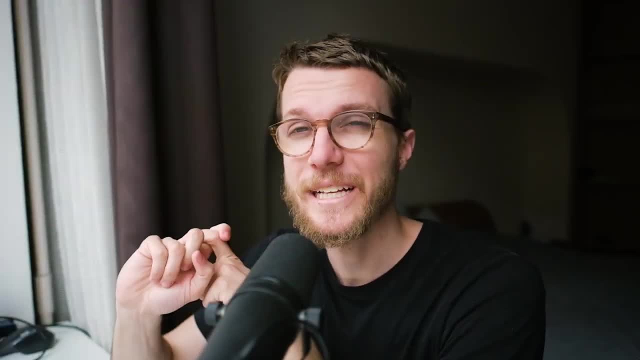 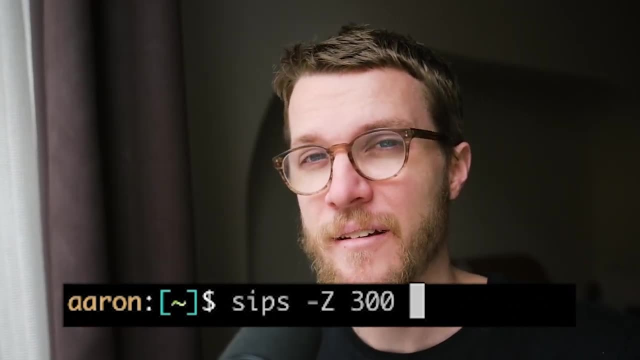 at a 300 wide resolution. Now there's a really cool way to make images smaller from the command line. You just use the sips z unix command. you pass in a wide pixel image and you're good to go With, for example, 300, and then the file name after it. Cool little trick for developers there. 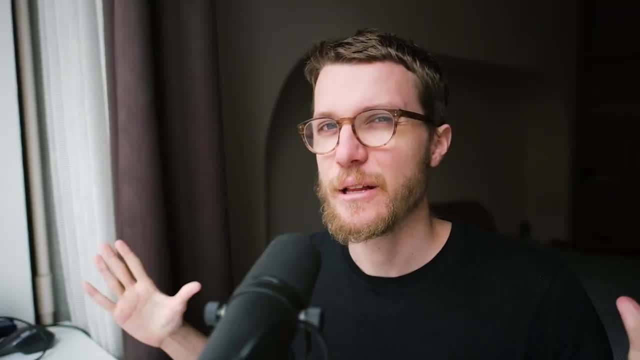 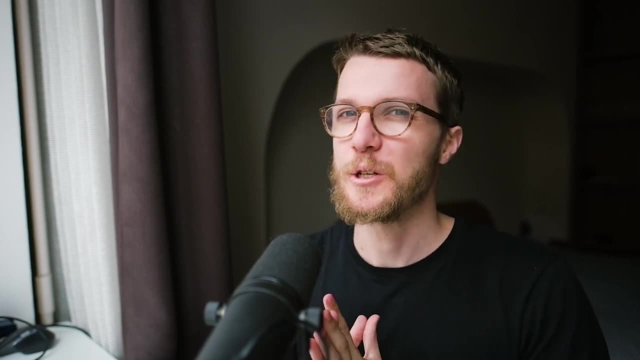 Okay. the next tip is to remove dependencies. A lot of developers out there just include jQuery and bootstrap by default, And these alone aren't huge libraries, but they do really add up when you combine them with everything else. I recently paid a freelancer to code a website. they were 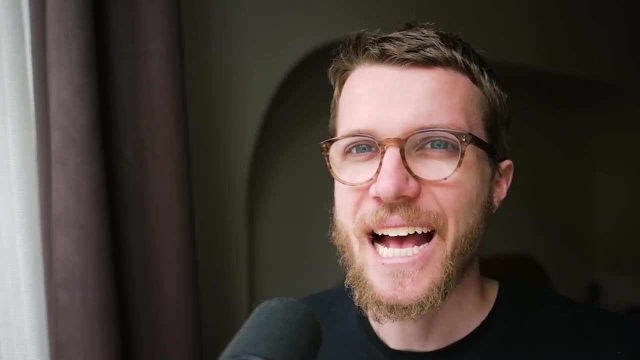 importing jQuery and only using it one time, And if you're building fast, simple landing pages, there's really no need for jQuery in most cases. Anyway, lighthouse and speed tests will usually tell you which libraries are the best for you And if you're building fast, simple landing pages. 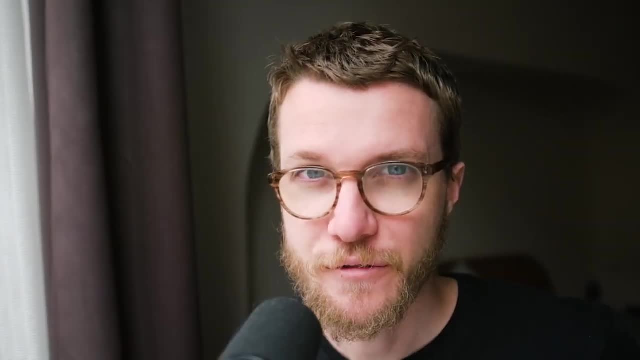 there's really no need for jQuery in most cases. Anyway, lighthouse and speed tests will usually tell you which libraries are the best for you And, if you're building fast, simple landing pages are barely being used, and give you suggestions on which ones you can remove. Okay, the next speed. 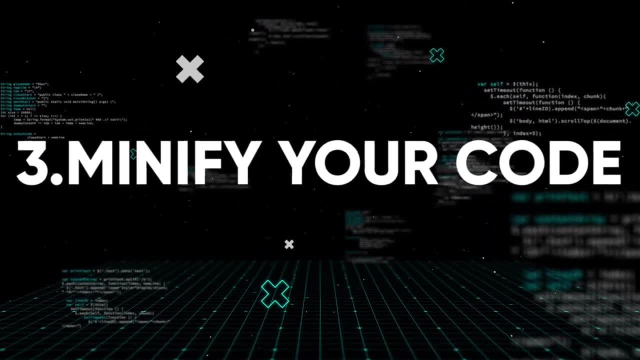 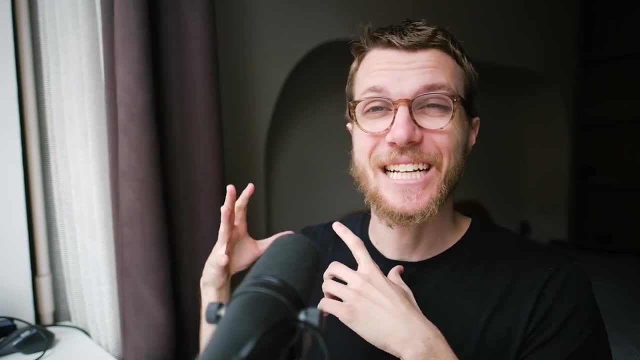 tip is to minify your code, And you can do this with a compiler or also online. Now, granted, this one won't have as big of an impact as the other tips because, frankly, code is not going to take up nearly as much space as an image would, but it all counts. So what you can do is also use 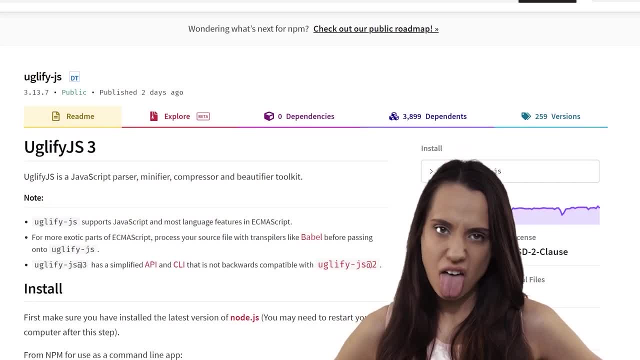 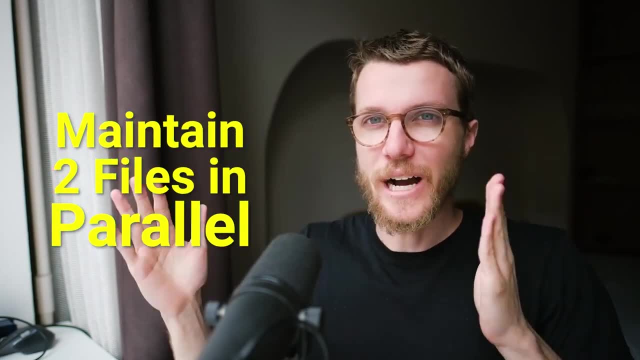 an online converter or an offline compiler to uglify your code or just make it condensed down into an unreadable format. The downside to this is you have to maintain two files in parallel and keep them updated. That is your readable code and your non-readable code, but it is something that's going to have a non-zero effect Next up. 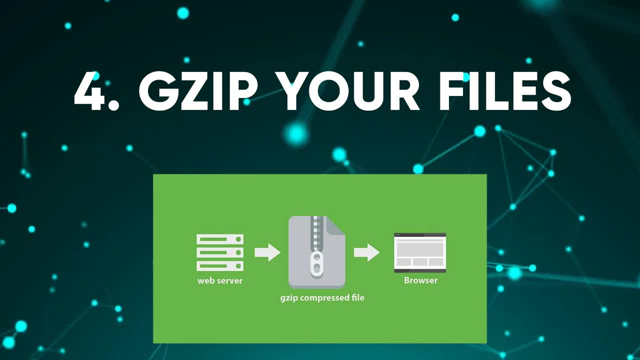 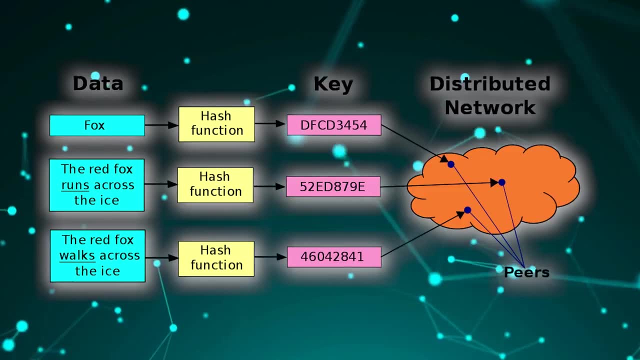 you can actually gzip your files, which is converting them to a different format, Without going too far into it. this is basically compressing your files into something like a hash table where there's keys that'll then look up different parts of the file. that needs to be. 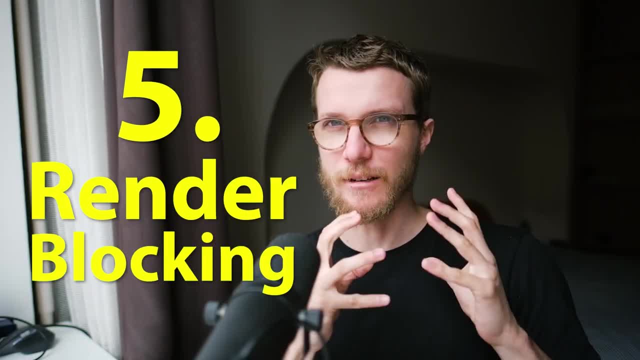 retrieved. Okay, number five: we want to reduce render blocking resources, And this would be of any non-critical asset on our page. So first, what does render blocking mean? Well, it's the things that need to happen before our page gets blocked, So let's go ahead and do that. So first, what does? render blocking mean? Well, it's the things that need to happen before our page gets blocked, So let's go ahead and do that. So, first, what does render blocking mean? Well, it's the things that need to happen before our page gets blocked, So let's go ahead and do that. So let's go ahead and. 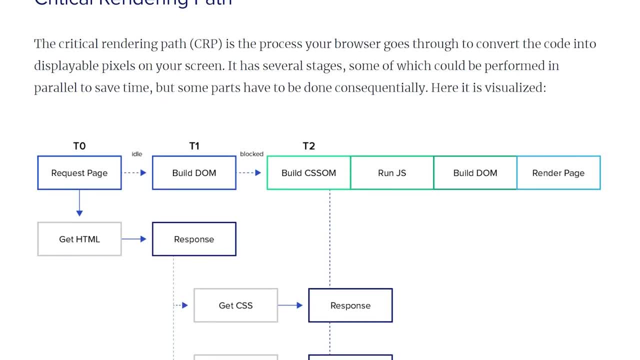 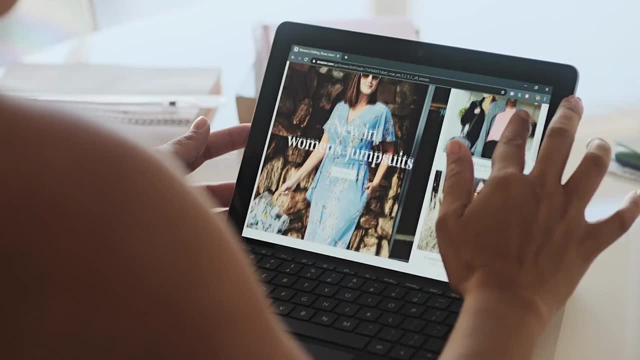 actually be fully loaded. And what about critical resources? Well, we usually consider these, any assets that are above the fold or on the top of the page before scrolling. Now, these are not really optional before the first paint, which is the first time things appear on the screen, Because 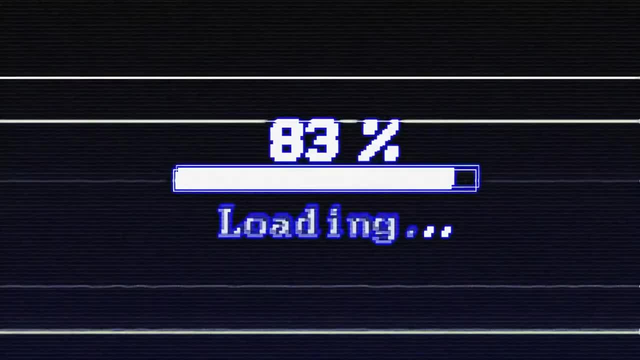 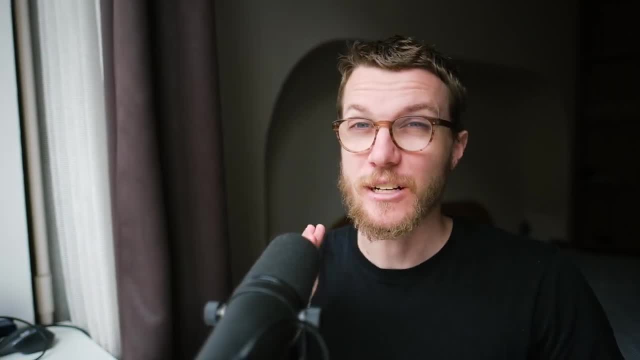 if we defer their loading, things are going to pop in and just look really bad. Now, this is okay for things further down the page because they have more time to load, And those are actually called non-critical assets And for each we do this in different ways. On scripts, we can put defer and 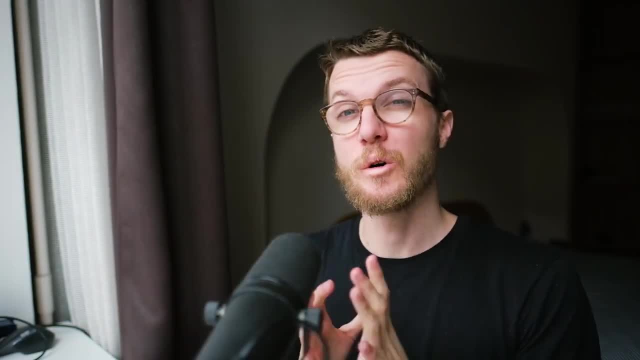 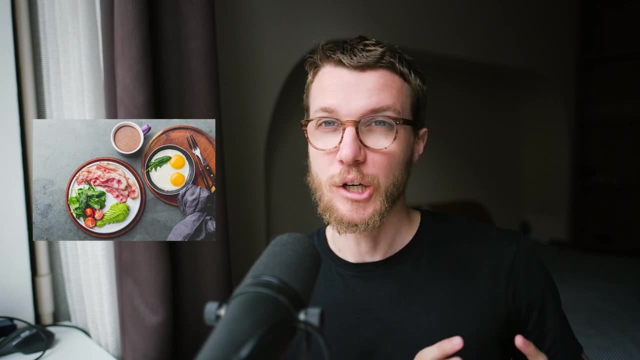 async. For CSS we have to be a bit more clever, And for images it's pretty cool. We can just put loading lazy in modern HTML. Of course, you can get deeper into it and have multiple versions of images, For example, a smaller one that loads first and then a larger one comes in. You can. 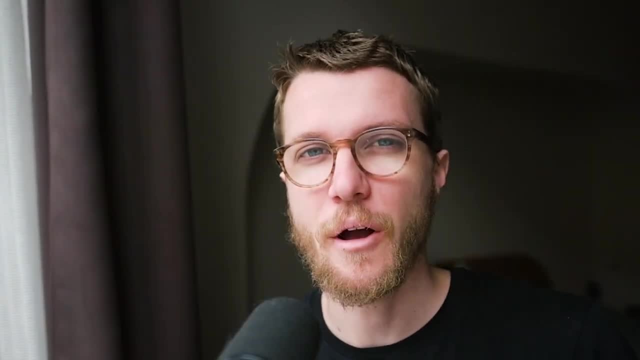 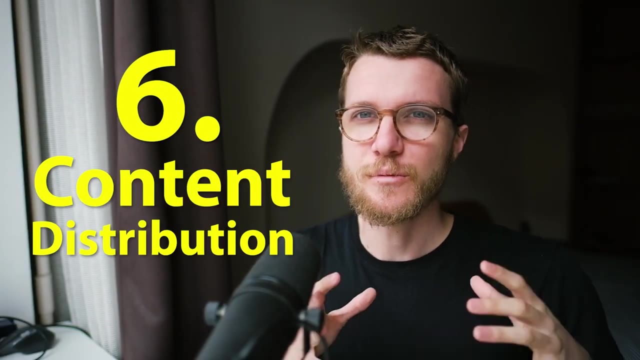 also have different image sizes for different resolutions. But let's stick to the simple low hanging fruit for now. Anyway, that was at least two different tips in there, So let's just make that two, Okay. the next tip is to use a CDN, or content distribution network. Basically, a CDN is: 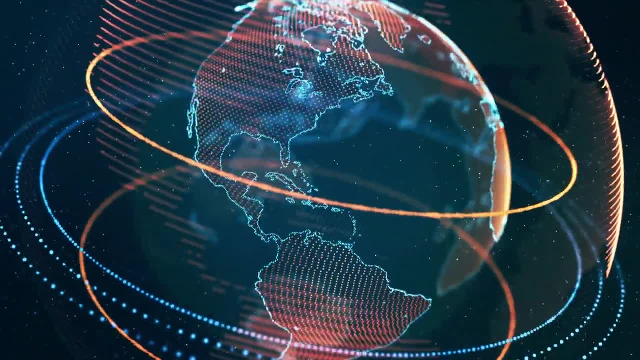 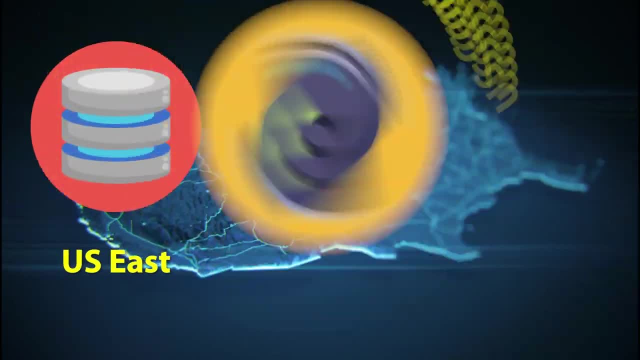 just different servers located around the world, And your asset will be loaded from the closest one to the request. Now, of course, you could say: well, I don't know, I don't know, I don't know, set this up yourself by creating, let's say, different AWS servers manually. There's also a 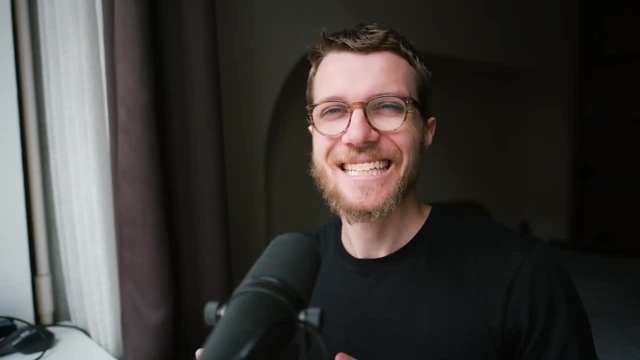 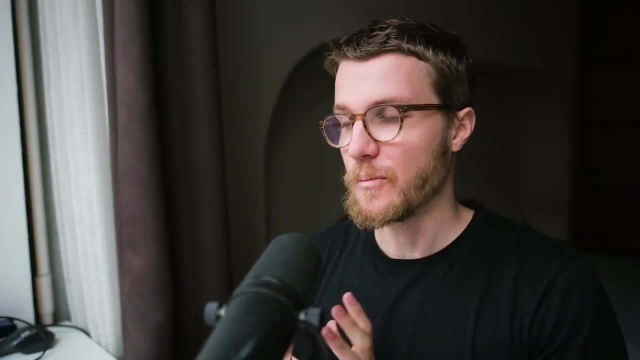 lot of services that do this for you, But the way you're going to usually do this in practice is using the CDN link of a library rather than downloading that code, Because if you download it, it will only come from your server. So best example is like jQuery. Again, you have a CDN link. and you have a download link. If you use that CDN link it'll most of the time just load faster than the downloaded code And you also don't have to deal with the complexity of downloading it, So it's usually the better option. 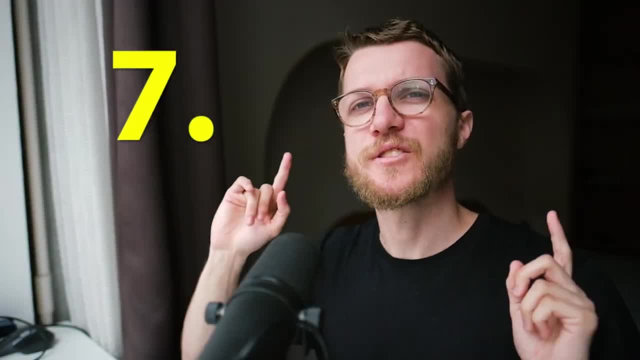 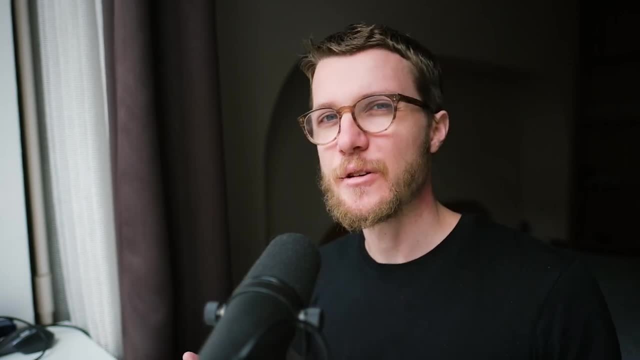 And you can do this with any asset. It can be libraries, it can be images, whatever Number seven is, using browser caching. Now, a lot of this happens by default, but you can slightly change the configuration to last longer, And you can do this by setting. 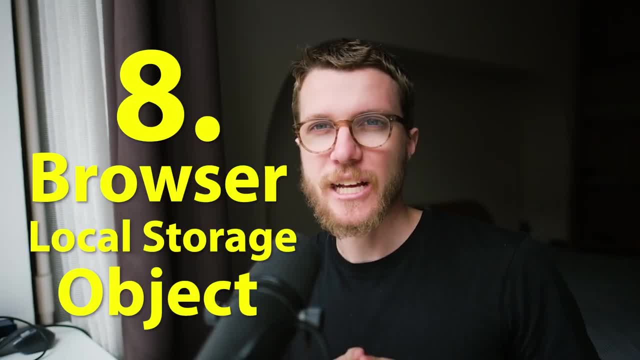 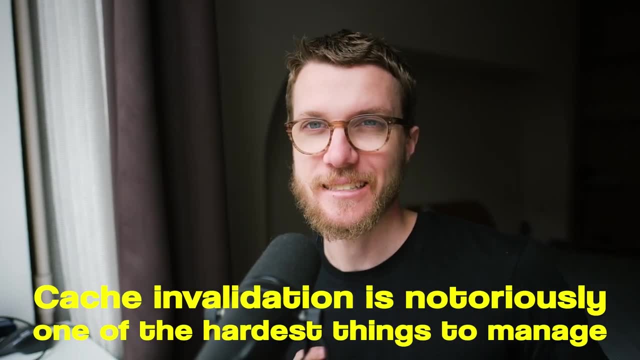 the cache control header, And you can also use the browser local storage object, though be careful, this is not very secure. You got to be a bit careful with caching, though, because cache invalidation is notoriously one of the hardest things to manage in programming. That is when 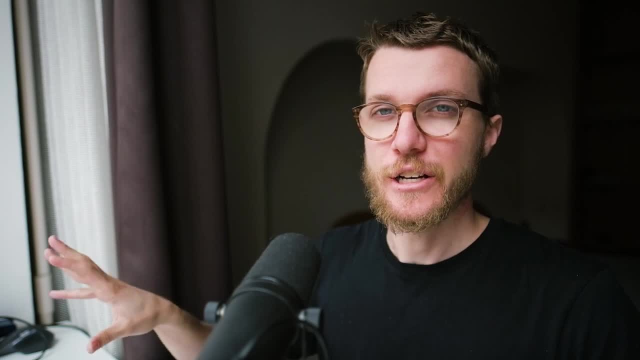 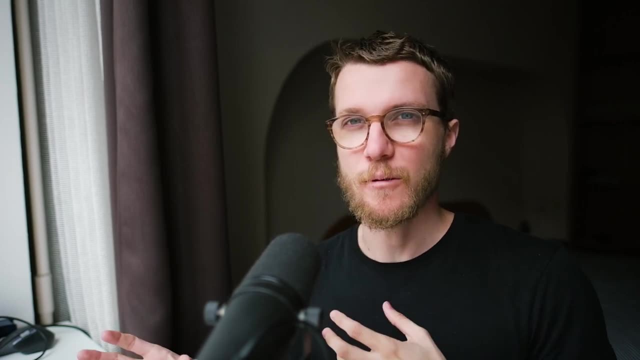 is your cache stale And when do you need to go back to the server for a new version of that file? This tip is kind of for advanced developers only, So if that doesn't sound like you, I would just make sure your cache isn't doing anything. 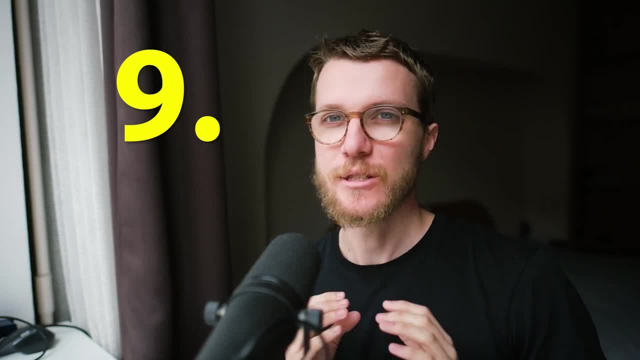 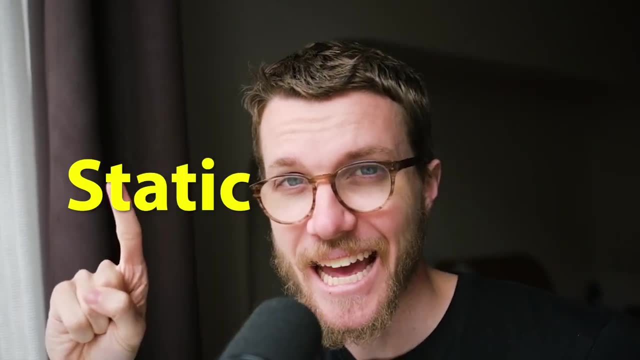 weird. I wouldn't worry about this one too much. Number nine: you can switch your site to using static pages. Now there are three main types of websites or web apps out there. The first one is static, And this is like traditional HTML, CSS, JavaScript. But now that a lot of things 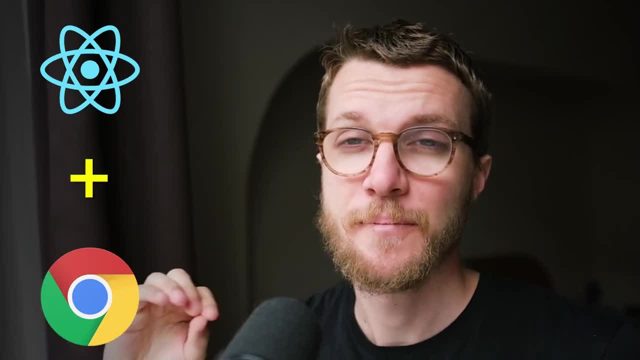 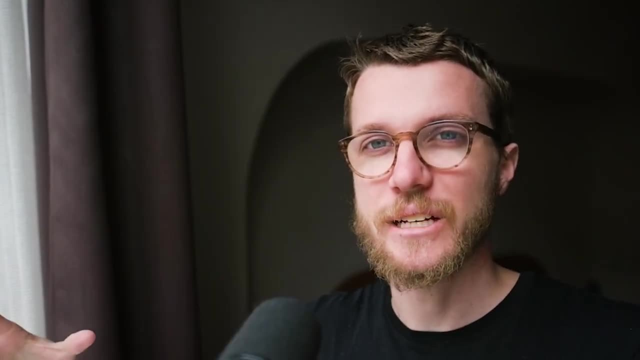 are done with frameworks. client side single page apps were created, which basically creates all of our HTML when we do the request using JavaScript, And this can actually dramatically increase the amount of time that we're going to be using JavaScript. So, if you're using JavaScript, you 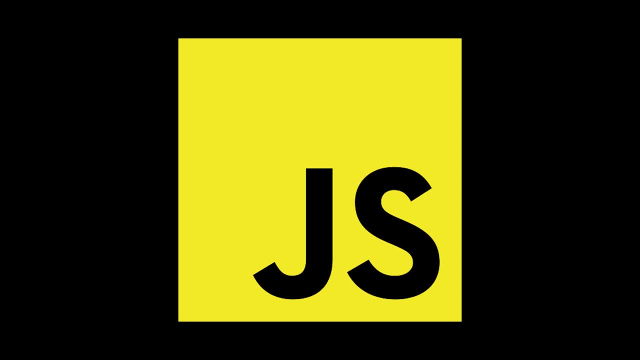 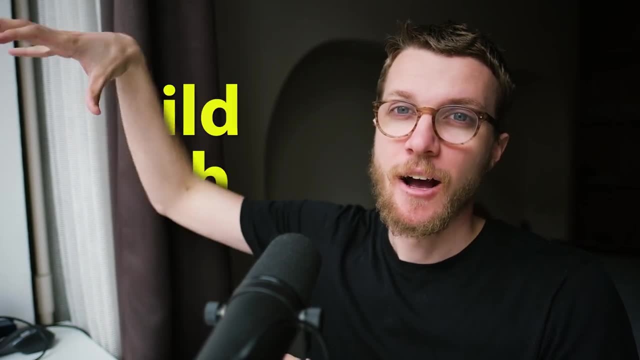 don't have to worry about the amount of time it takes your site to load if we have a lot of JavaScript or a large bundle. And then there's a third type called server side rendering, where this same build with JavaScript thing will happen on our server and then it'll send that. 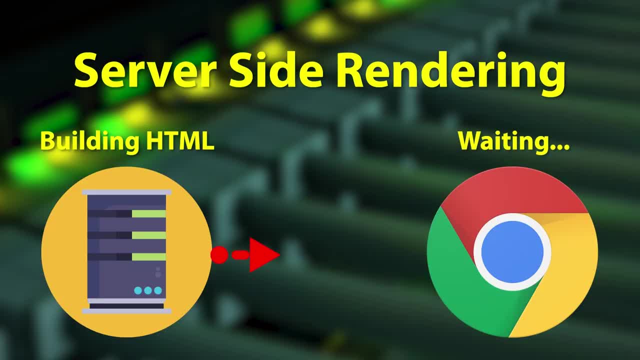 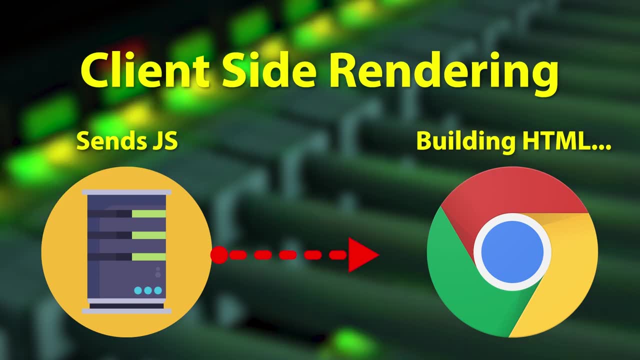 build code to the client. So the difference is it's going to take us longer to receive our first byte. if we're building things on the server And with client side rendering, we'll get our code faster, but it still has to load on the client. Now, if static pages are faster, why would you?